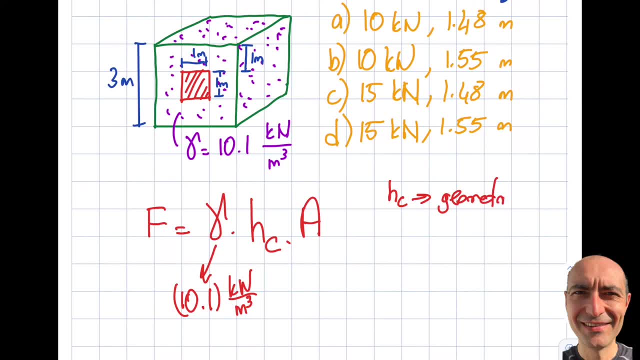 this is an example of an example of a newton and this is an example of a HC. is for the geometric center, okay, and this is not the where the pressure is acting on. okay, this is if you want to think about it. this HC is in the easier. 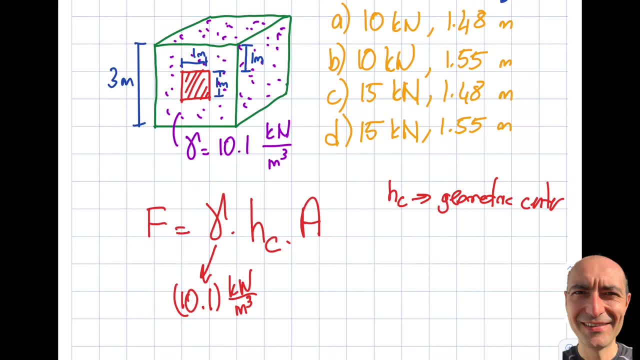 end of the spectrum, okay, and if I'm asking you H, or we call it Y, YCP or central pressure, then it's on the harder end of the spectrum, okay. so let's not confuse them, because I'm still using like a pressure and sometimes I see 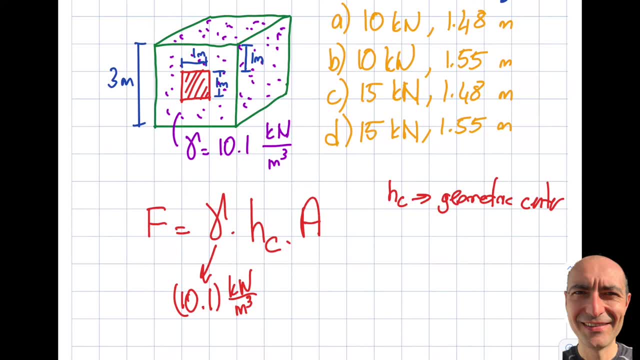 students using central pressure in here. that's not quite accurate. okay, it's easier than that. so I'm looking at this particular shape rectangle. that will be the well I'm indicating, actually, when I'm asking a question. that will be the center of the geometric center of this plate. it will be right halfway through. 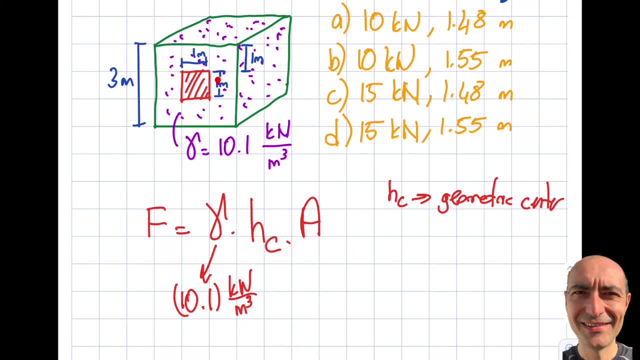 it right. so if you think about it, it will be halfway through it. so this will be 0.5 and you see what is given here. 1 meter, 1 plus 0.5 is 1.5 meters. that's what I'm gonna get for my HC value. what about the area? 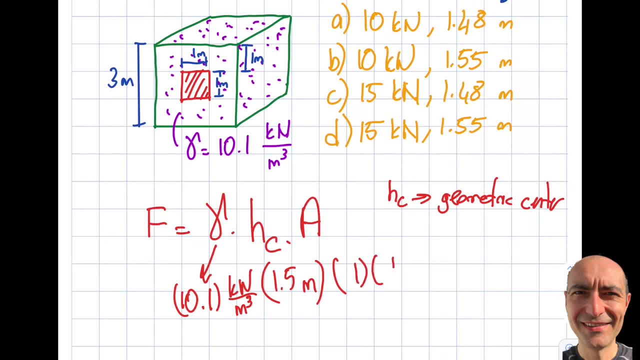 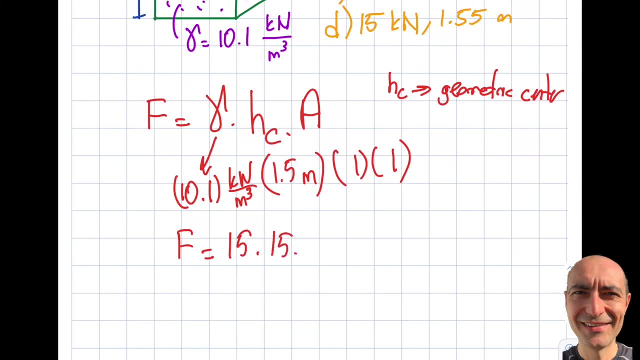 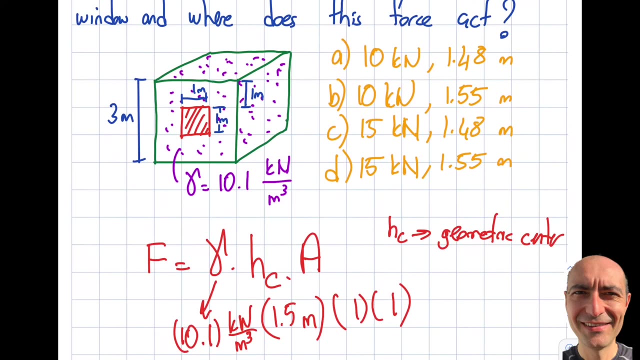 well, it seems easy. one is the width of it, one is the height of it and from here I will get my F to be 10, 15 point 150, right. 50 kilo newtons, right. so when I look at the choices you can see that I'm down to C or D, right. AB is out, okay. so. 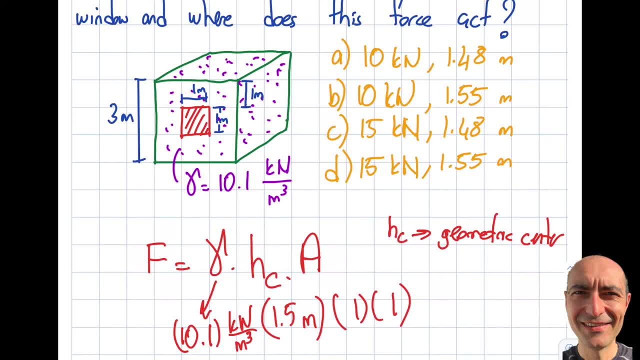 that's good. that's something, by the way. I'll tell you a little hint. this is very handy and I mentioned this multiple times, but it's important to repeat because we know my repetition is this: the center of pressure will be a little bit lower in terms of the absolute sign it will be. 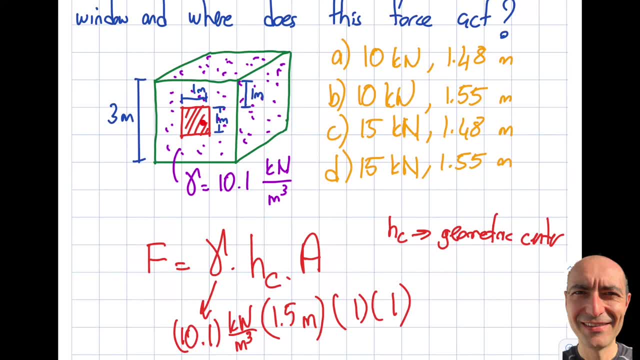 higher number, okay, but in terms of the location will be a little bit lower than the HC value. let's say that the HC is right here. this HC YCP will be a little bit lower than that, okay. and so when I look at the choices that I have here and you do realize that this HC was 1.5 and one of 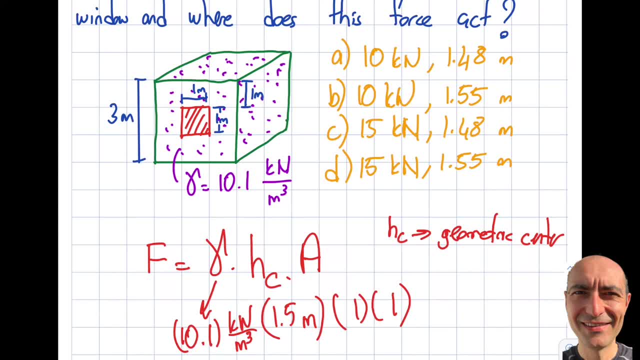 the choices 1.48, so the right answer is D. okay, so you can use this. and on the real exam questions, I have observed that this logic sometimes gets easier of the 3 out of 4 answers okay, so this is very important. so I would like 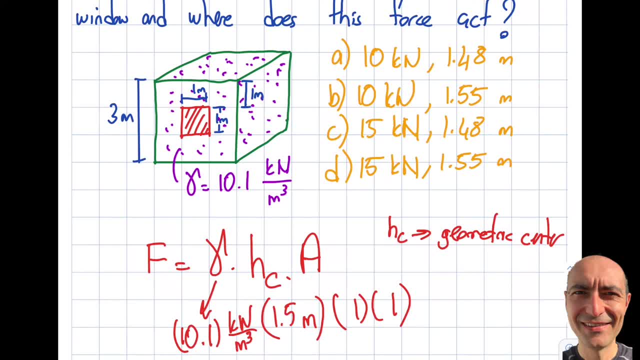 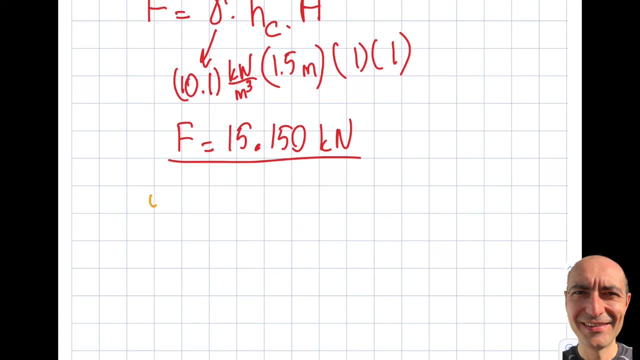 you to be cognizant of that right. but let me show you how to do it because, well, who knows, maybe you would be, you're gonna need it. right, there's a formula for that. so Y C P will be equal to Y C plus I X C. 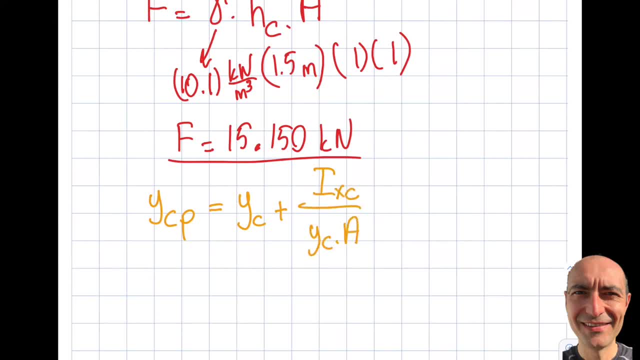 divided by Y C times a. so where did I just get this from? it looks complicated. did I memorize this? no, there's something called a fee reference manual, right? you're looking at it right in front of your screen. there are two screens. one screen has it right, so you have access to this formula, and it's on page 179 for. 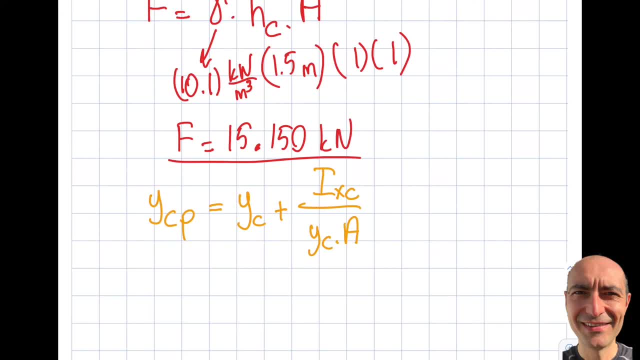 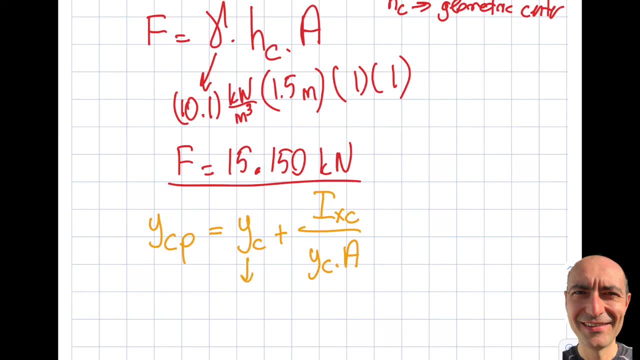 the 10th edition of this, you know, reference manual. ok, and what they say about this YC is: I want to be clear on that one. this is 1 point 5. ok, so they're talking about this value. one point five. this is one point. 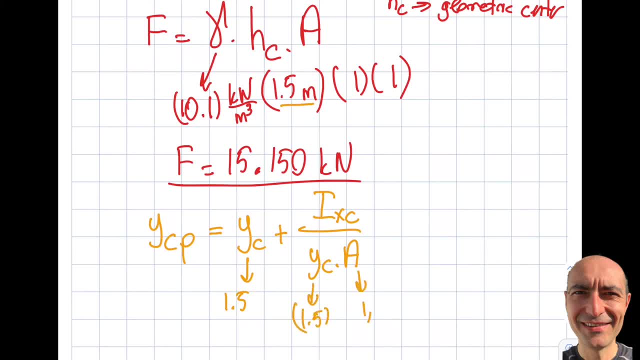 five, what about the area balance up there? so the good thing about one time- smile- the good thing about this is that you kind of have only one term missing over here. if you do the approach properly, you will only have this term. dressed will already be analyzed, ok, you. 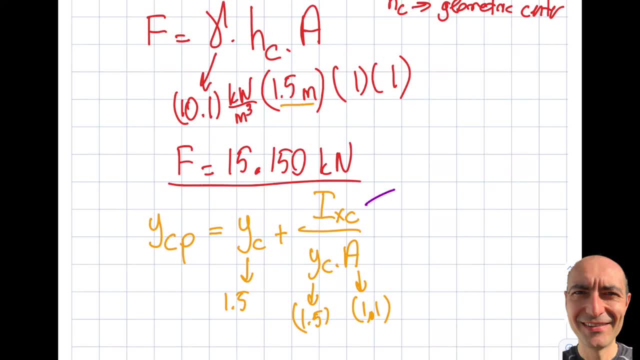 you come to here IXC, I need to. this is unfortunately not written, at least in the fluid mechanics section of it. okay, but for simple geometries like this you may want to memorize this and I'm sure many of you now is valuable. you're watching this video is telling me this: 1 over 12 times BH cube. okay, B is the. 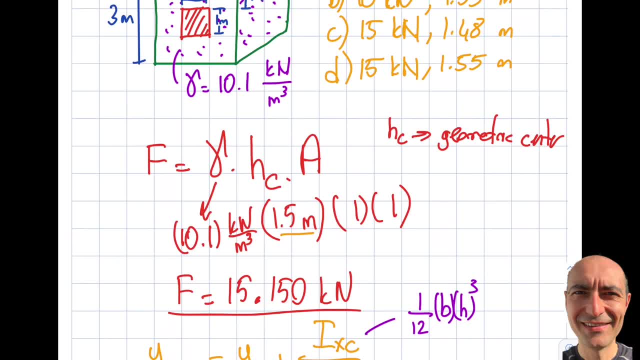 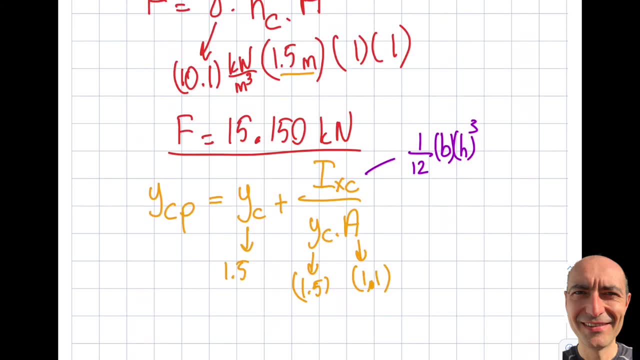 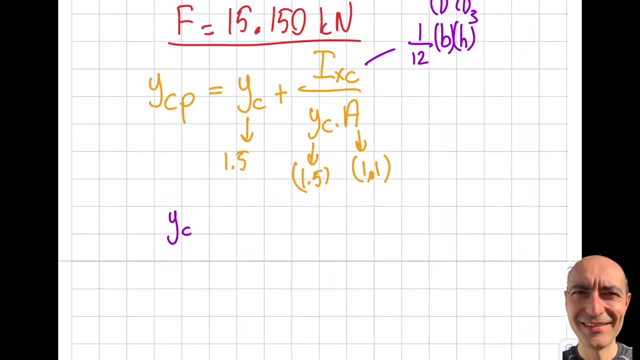 base. okay, so let me show here: the B is the base and height is 1. in this case it doesn't really matter, right, but still it's important to notice that from here this will be 1 times 1 cube, okay, so then you can see over here what I get is Y CP. 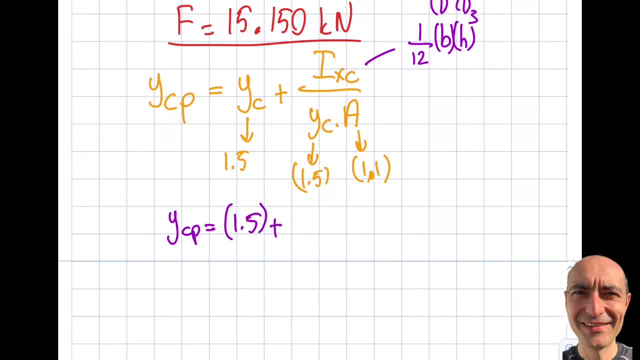 is equal to 1.5 plus what did I say? it will be a little bit more than that, right? that's why there's a positive sign. I'll get myself 1 over what is 1.5 times 12. that is 18, right? so you can see, it's a little bit more than 1.5, and I'm sure. 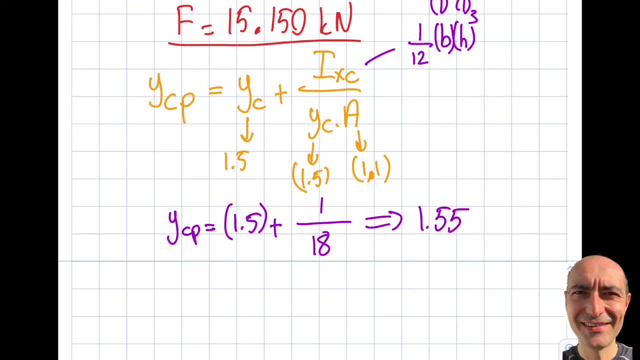 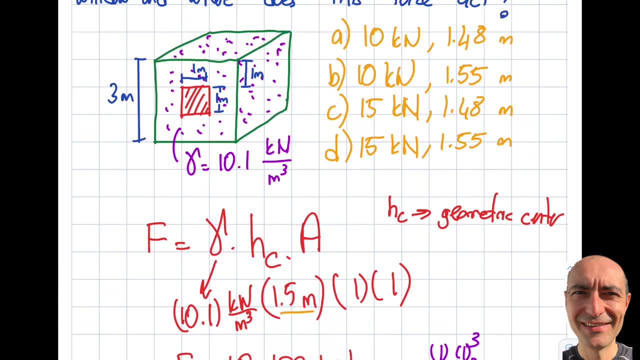 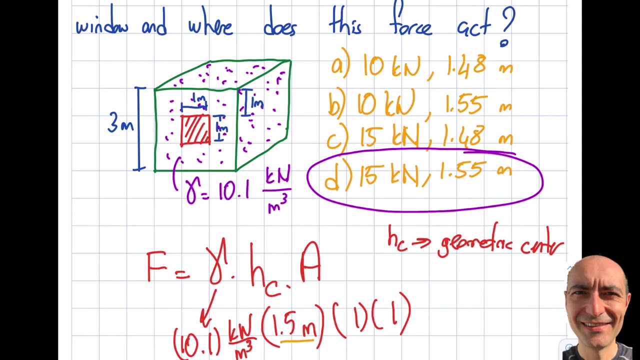 it's gonna be right around 1.55. okay, actually one. it should be like this, right? yeah, okay, so this will be meters, this will be. you see, it's a D is the closest one that I get. thank you for watching this video. okay, let's go one step higher than the previous question. 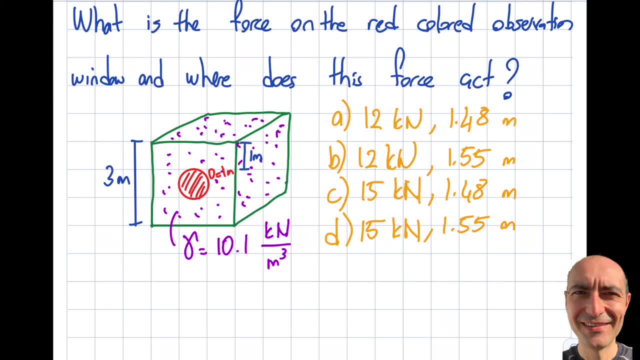 okay, back then, do you remember that I had this as a rectangular observation window? right, this was a rectangular case. right now, this turns out to be a circular one. okay, an observation window. and I'm asking you: what is the force? and I'm asking you what is, or where is it acting? the first thing is, the formula is the same, so 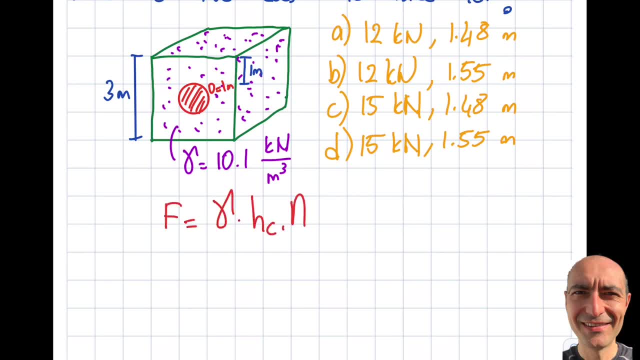 again I mentioned- you should memorize this right. this is 10.1 kilonewton per meter cube. HC is still 1.5. let's talk about it for a second. the center of the, the location of the geometric center, is right at the center of the. 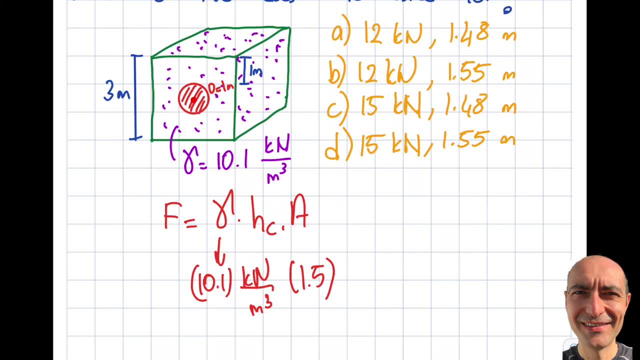 circle cross-section. right, but you can see. so that means 0.5 up here, but there's also one here, so it becomes 1.5. so this is identical to the previous question. okay, how about the area? so the area itself will be pi R square or pi D. 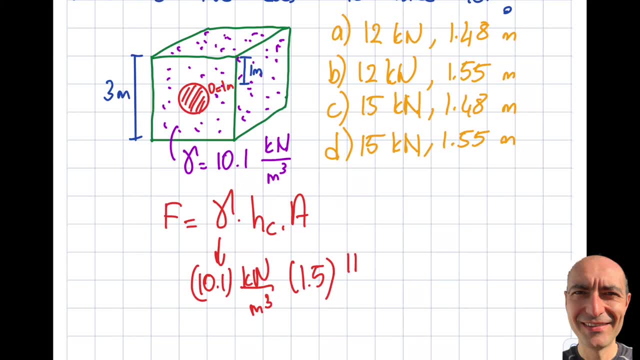 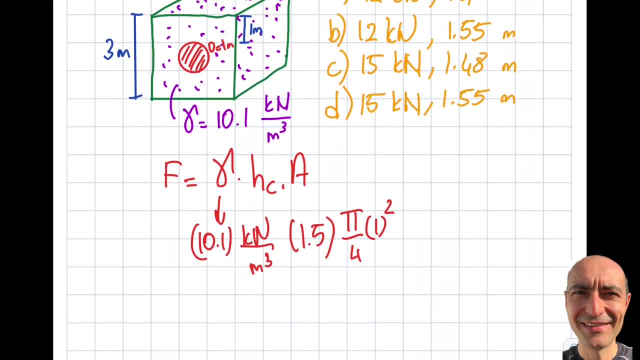 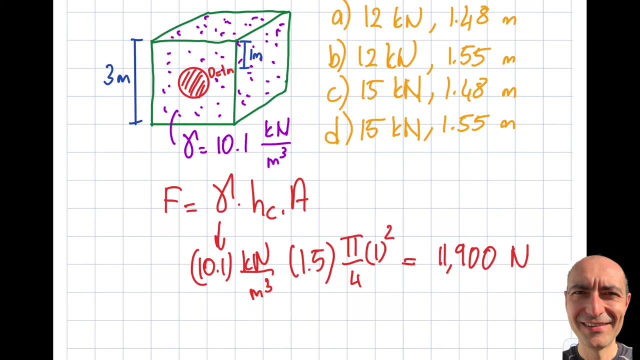 square over 4, right? so D is 1. so let's write it this way: pi over 4, 1, square, right, okay? so if I punch this into my calculator, I will get myself a Newton's right. so it's right around this 12 kilonewtons range. okay, then let's go. 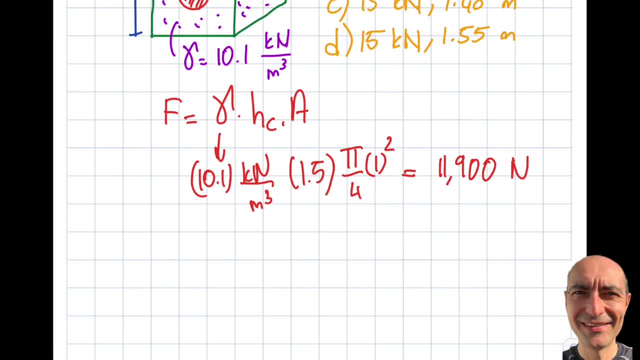 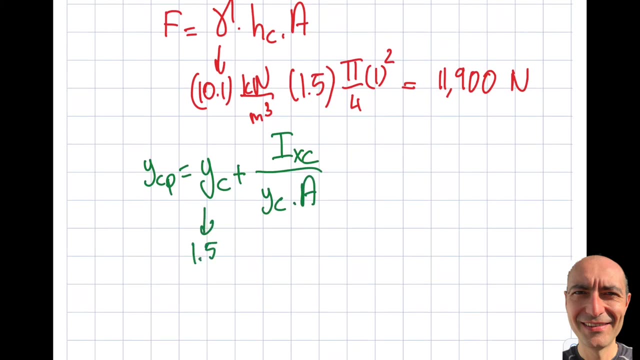 ahead and find where is this acting. okay, and it's the same formula as the last time, so I'm gonna get myself. Y CP will be equal to Y C plus I X C divided by Y C times a right Y C is 1.5. this is 1.5. a raise pi over 4 up there, right what?